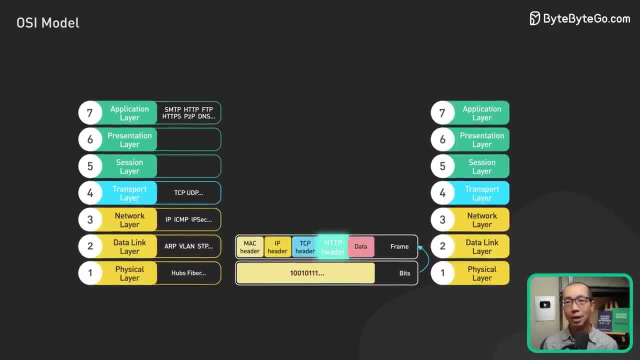 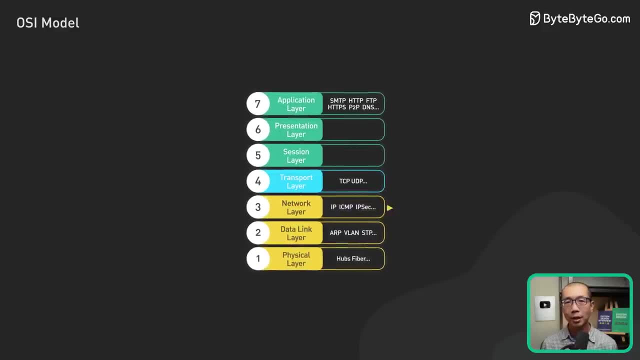 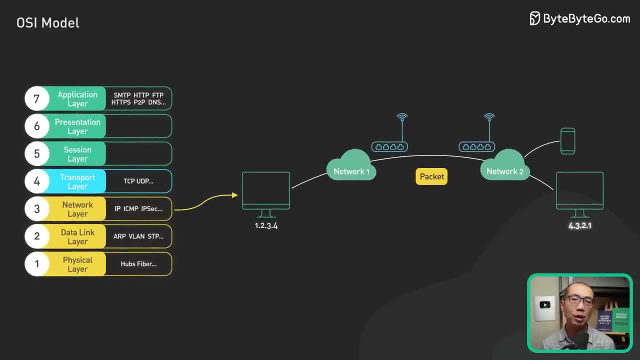 It ensures that the frames are delivered to the correct destination. The Ethernet primarily lives in this layer. The network layer is the third layer. It is responsible for routing data frames across different networks. The IP part of TCP IP is a well-known example of this layer. 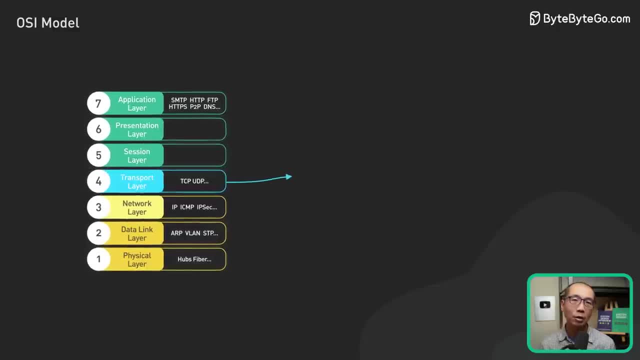 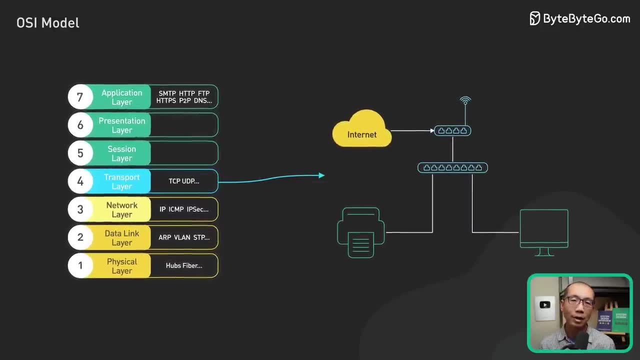 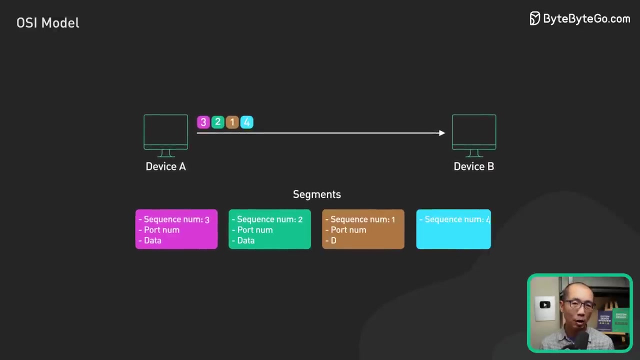 The transport layer is the fourth layer. It handles end-to-end communication between two nodes. This is the layer where TCP and UDP live. TCP provides reliable end-to-end communication between devices. It does this by dividing the data into small, many layers. 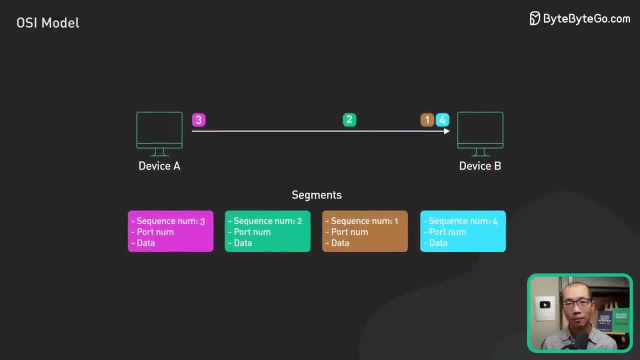 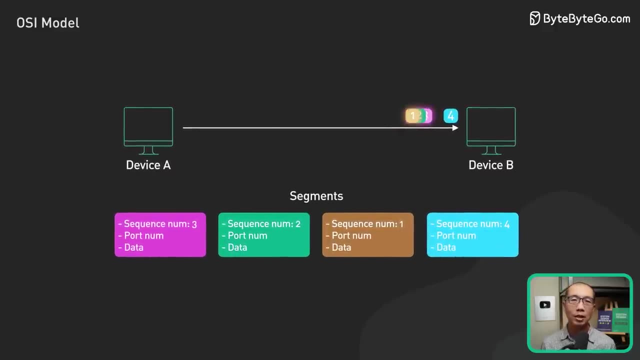 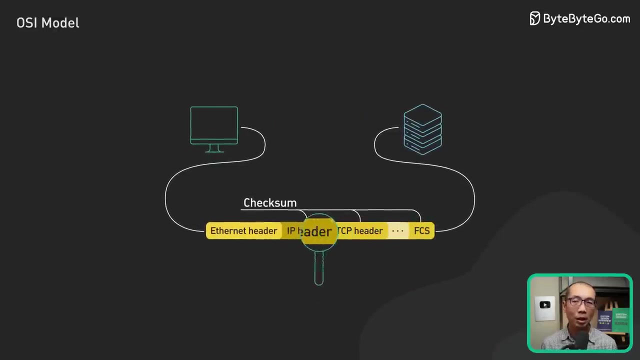 It is a very simple way to manage both segments and sending each segment individually. Each segment has a sequence number attached to it. The receiving end uses the sequence numbers to reassemble the data in the correct order. TCP also provides error checking to make sure that the data was not corrupted during transmission. 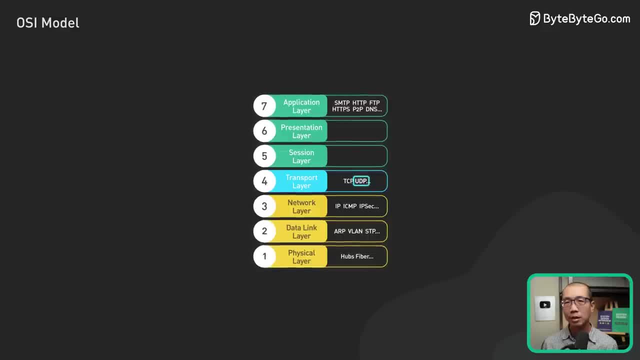 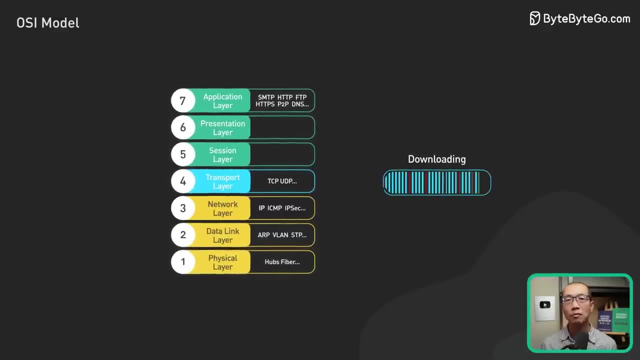 UDP is another popular protocol in the transport layer. It is similar to TCP, but it is simpler and faster. For TCP, UDP does not provide the same level of error checking or reliability. It simply sends packets of data from one device to another. 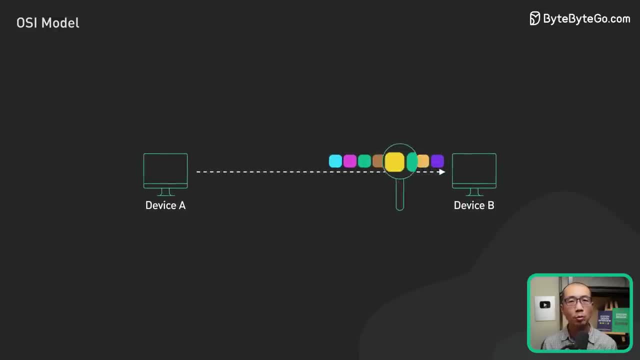 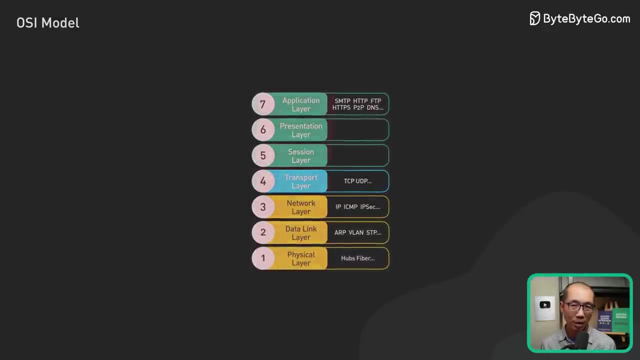 The receiving end is responsible for determining whether the packets were received correctly. If an error is detected, the receiving end simply discards the packet. The remaining layers are session, presentation and application layers. This is where the OSI model loses its usefulness in practice. They are too fine-grained and do not really reflect reality In general, it is sufficient to collapse them into a single layer and consider application protocols like HTTP as simply layer 7 protocols. Let's go through an example and examine how data moves through the layers. 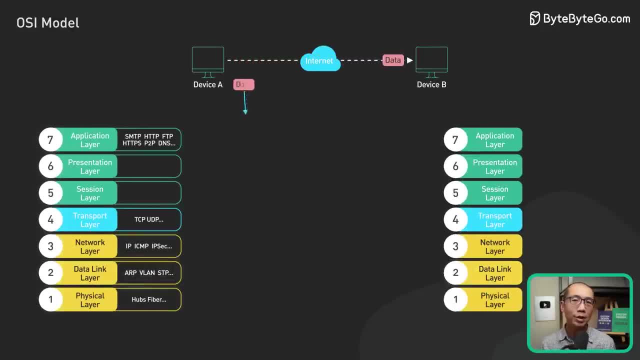 when transmitting over the network. When a user sends an HTTP request to a web server over the network, the HTTP header is added to the data at the application layer. Then a TCP header is added to the data at the application layer. It is encapsulated into TCP segments at the transport layer. 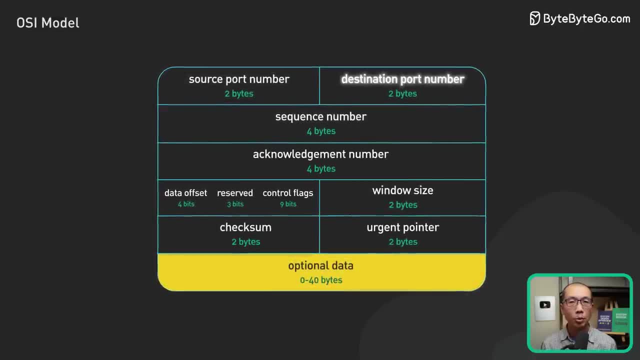 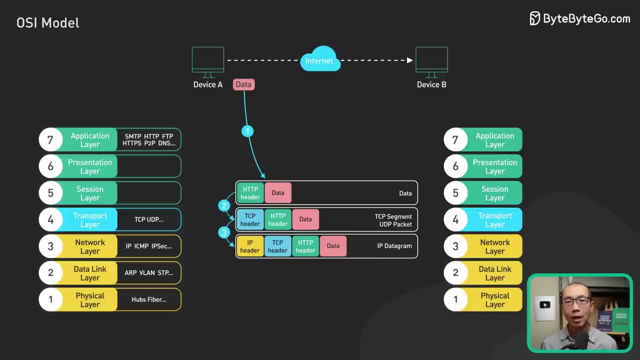 The header contains the source port, destination port and sequence number. The segments are then encapsulated with an IP header. at the network layer. The IP header contains the source and destination IP addresses. A MAC header is added to the data link layer. 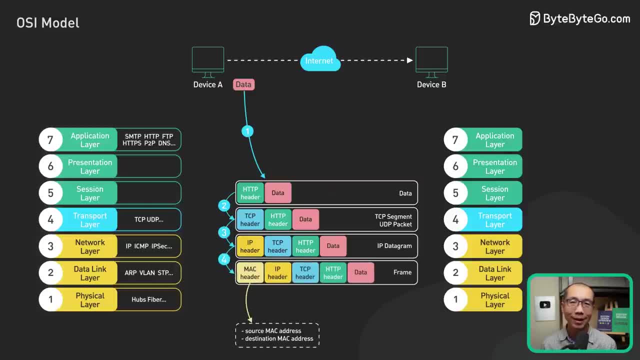 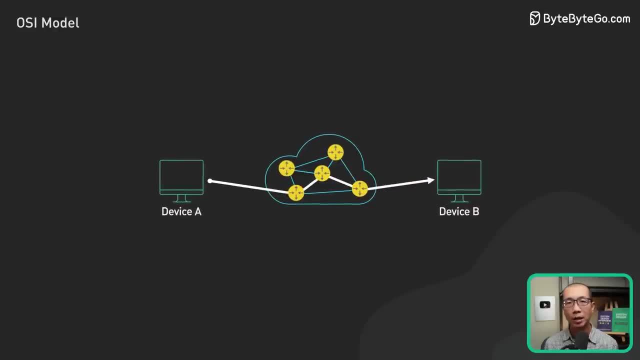 with the source and destination MAC addresses. It is worth noting that in the real world this is a bit nuanced. The MAC addresses are usually not the MAC address of the sending and the receiving ends. They are the MAC addresses of the routing devices in the next hop.